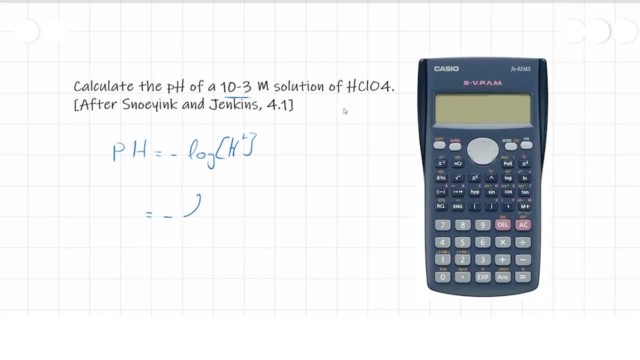 This means I have: pH is equal to minus log 10 to the power minus 3.. To be able to use the calculator to calculate this formula, I click first the minus, then the sign of the log, then I write 10, then this sign, which is to the power minus 3.. 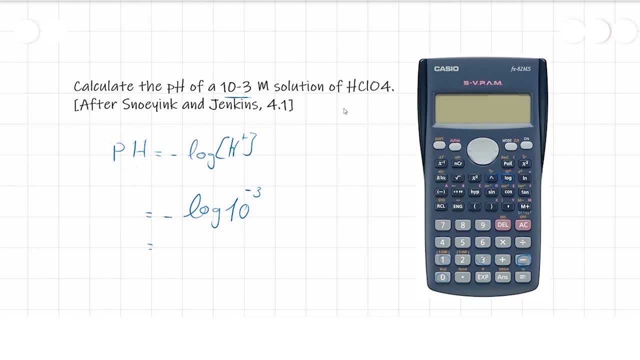 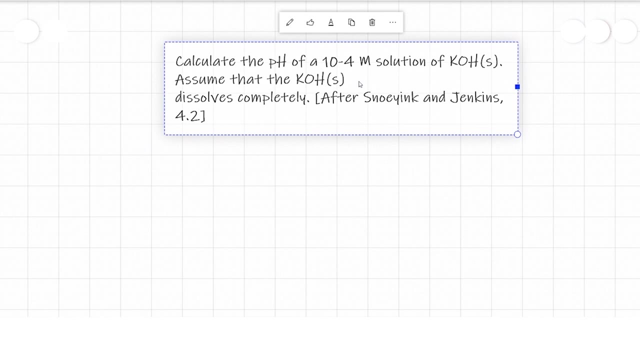 I click again the minus, then I click the 3.. Finally I click equal. This will give me that the pH of perichloric acid is equal to 3.. Okay, Calculate the pH of 10 to the power minus 4. molar solution of potassium hydroxide. 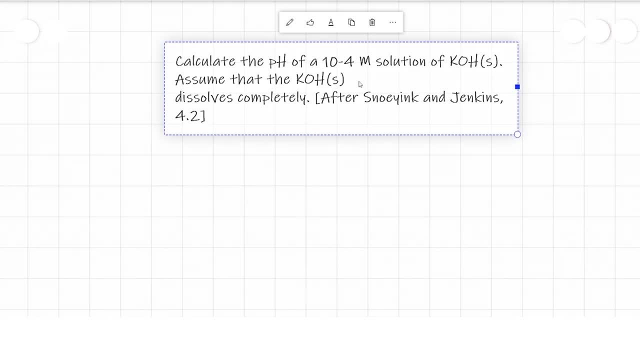 Assume that the potassium hydroxide solid dissolves completely. So we said that pOH is equal to minus log, the OH concentration of my solution. In here I have it: 10 to the power minus 4.. So the pOH is equal to minus log, the OH concentration of my solution. 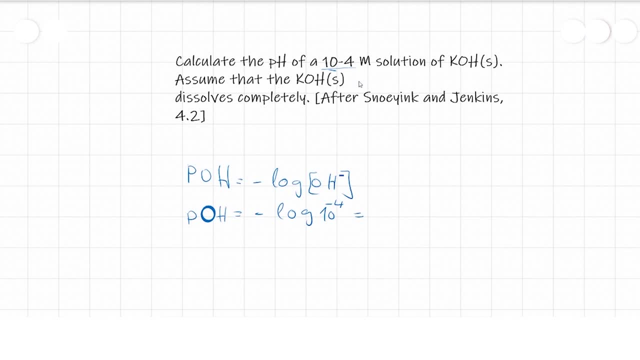 This is equal to minus log 10, to the power minus 4, which is equal to 4.. I need the pH, not the pOH. This means that we know that the pOH plus pH is equal to 14.. So the pH is equal to 14 minus the pOH, which is equal to 4.. 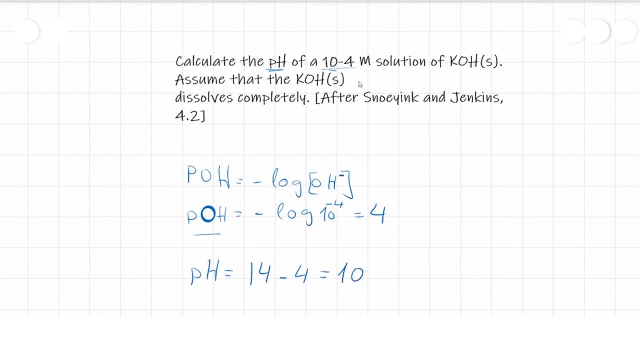 This will give me that the pH of my solution is equal to 10.. Acetic acid is a weak acid. The pKa is equal to 4.26.. If 10 to the power minus 3 is equal to 4.26.. 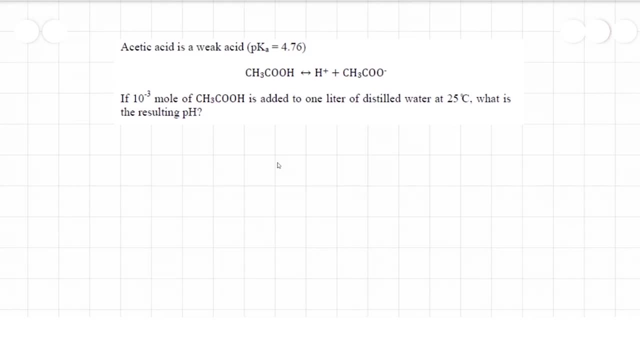 Then I have 10 to the power minus 3.. So I have 10 to the power minus 3.. If 10 to the power minus 3 moles of acetic acid is added to 1 liter of distilled water at 25 degrees centigrade. 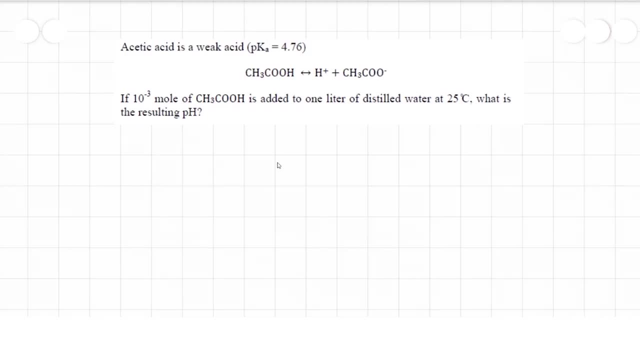 What is the resulting pH? First, let's write the equation: CH3- COOH in equilibrium with the hydrogen ions and the acetate ions. I have initial concentration In here. I have 10 to the power minus 3, which is 0.001, and I have in that case, the hydrogen. 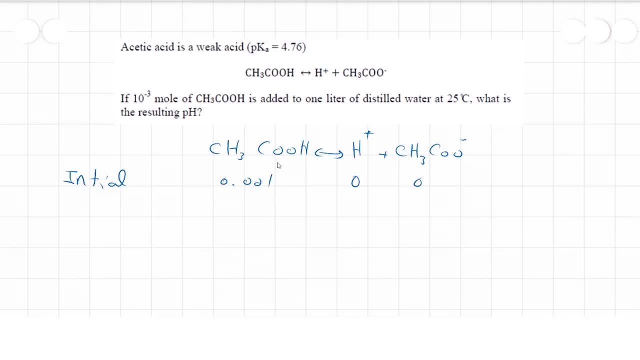 ions will be 0 and the acetate ions in the initial concentration will be equal to 0. That change, I will assume. in here it is minus X, in here it is X, and in here it is X as well. Now the final concentration would be equal to 0.001, minus the change that happens the 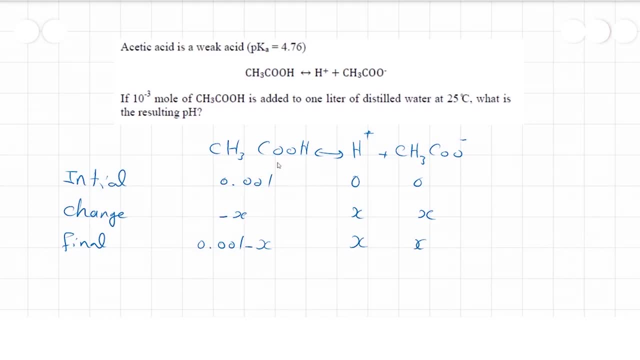 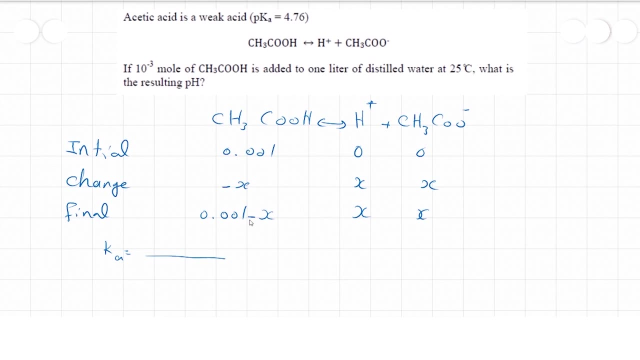 X. We know that the pA is equal to the concentration of the product divided by the concentration of the reactant. So I have hydrogen ions multiplied by the acetate ions divided by the acetic acid concentration, I have that the pKa's concentration is equal to II. 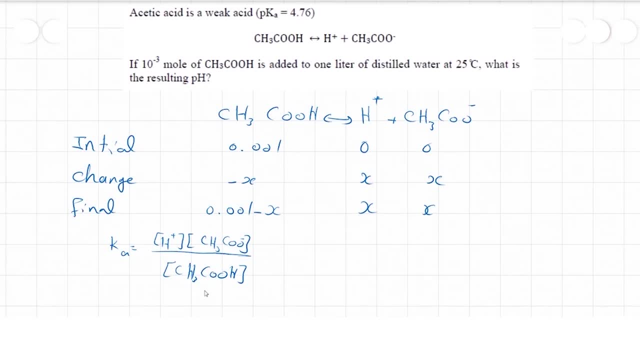 reactant concentration. Okay, In time, Okay. ke value is equal to minus log ke value. this means ke value is equal to 10 to the power minus pke value, which is equal 10 to the power minus 4.76. this will give me that the ke value. 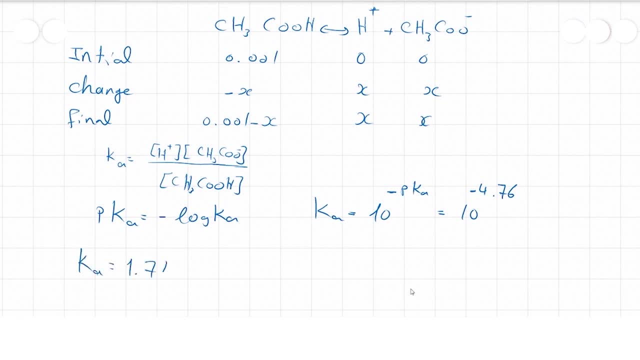 is equal to 1.74 multiplied by 10 to the power minus 5, the ke is equal to the final concentration of hydrogen ions, which is x multiplied by the final concentration of the acetate ions, which is equal to x divided by final concentration of the acetic acid, which is: 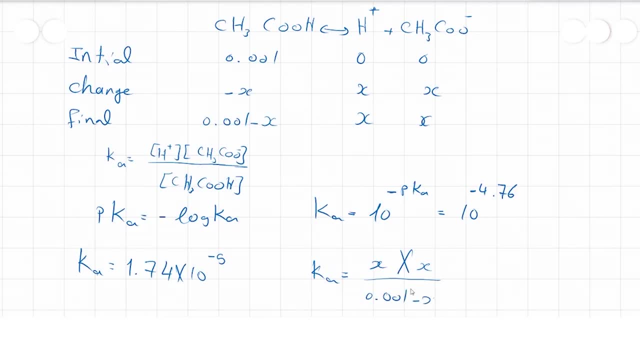 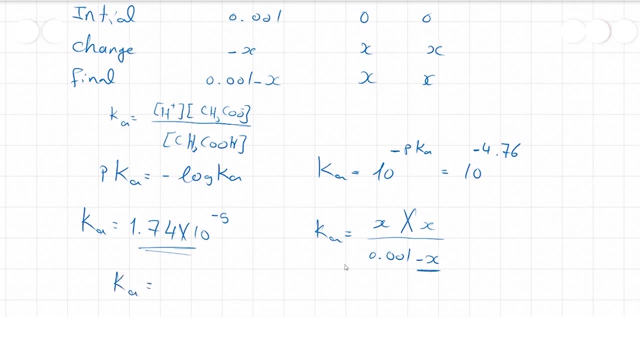 equal to 0.001 minus x. because i have a very small ke value, i will ignore the minus x. this means ke would be equal to x squared divided by 0.001. i have the ke value, which is equal to 1.74 multiplied by 10, to the power minus 5. 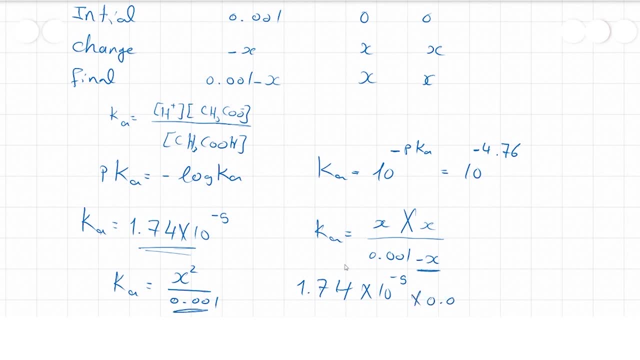 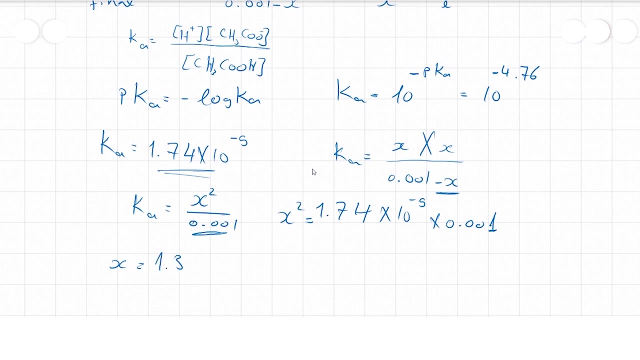 multiplied by the 0.001, this will be equal to x square. if you take the square root of this formula Now, this will give me that x is equal to 1.32 multiplied by 10 to the power minus 4.. Now I have that the pH value is equal to minus log x. 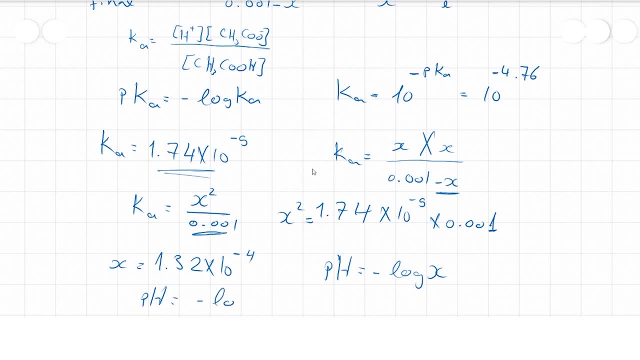 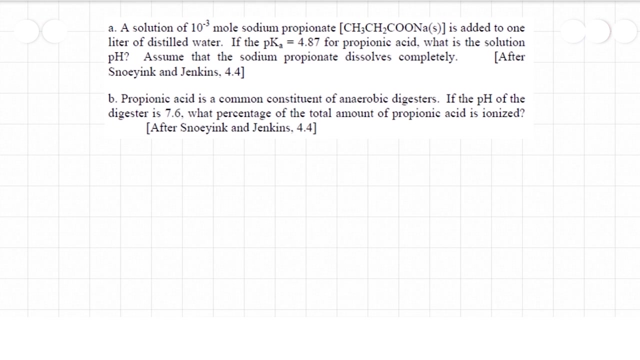 This means the pH is equal to minus log. this value, 1.32, multiplied by 10 to the power minus 4, is equal to 3.88.. The solution of 10 to the power minus 3 moles sodium propanoate is added to 1 liter of distilled water. 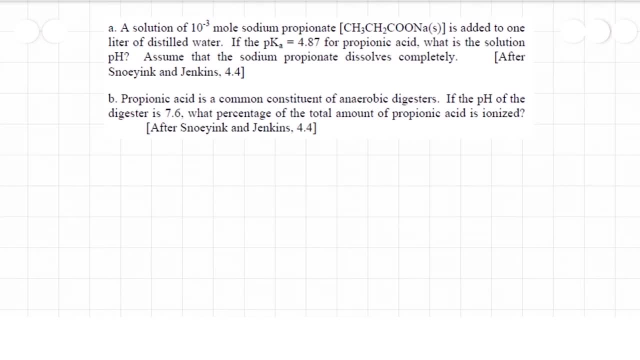 If the pKe is equal to 4.87 for propanoic acid, what is the solution pH? Assume that sodium propanoate dissolves completely. Propanoic acid is a common constituent of anaerobic registers. If the pH of the register is equal to 7.6,. 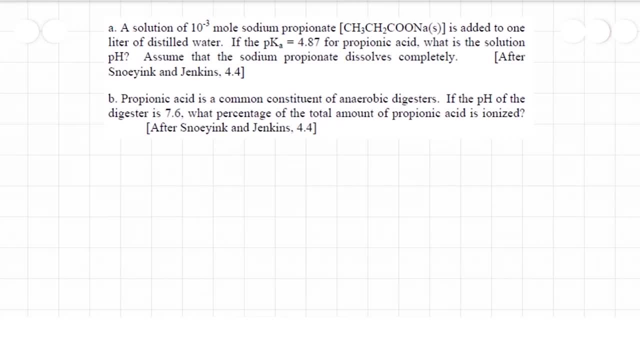 what is the percentage of the total amount of propanoic acid which is ionized? Let's try to write the equation. I have CH3, TH2, TOO Na, plus water will give me TH3, COOH. 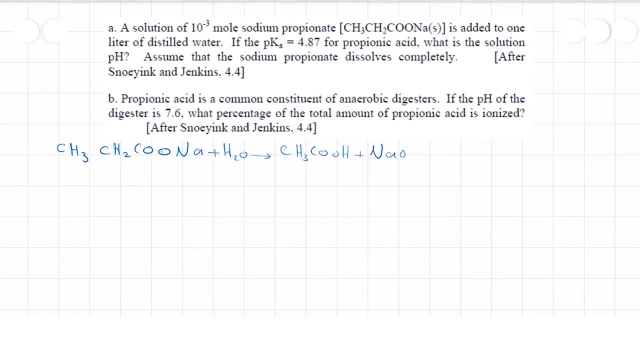 plus water will give me NaOH. The initial concentration of sodium propanoate is equal to 1 to the power minus 3.. We will ignore the concentration of water until I assume it is equal to 0 and here is equal to 0.. 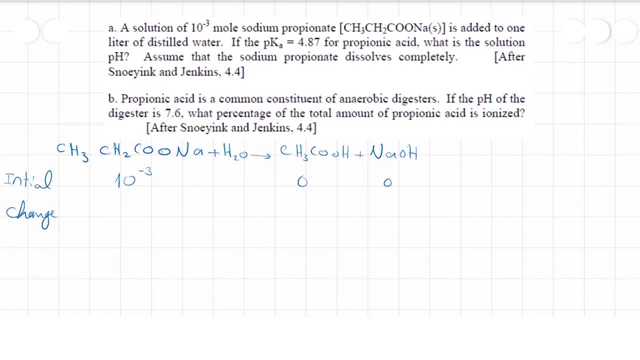 That change will be equal here to minus x, here plus x and here plus x. Finally, the final concentration will be T to the power minus 3 minus x, and here will be equal to x and x. I have: p is equal to x squared product divided by the reactant: T to the power minus 3 minus x. 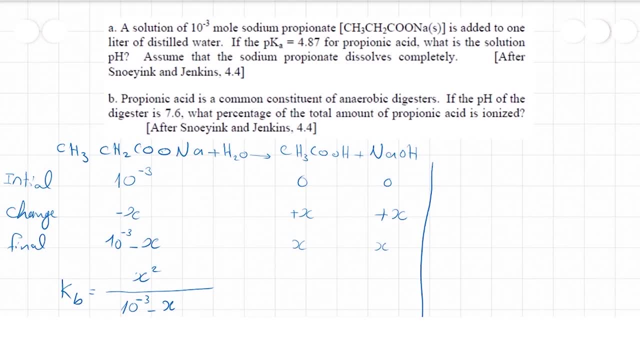 First we need to calculate the value of p, because here we have the value of the value of p. We know that pk plus pkp is equal to 14.. This means pkp is equal to 14 minus the value of pk, which is 4.87, equal to 9.13.. 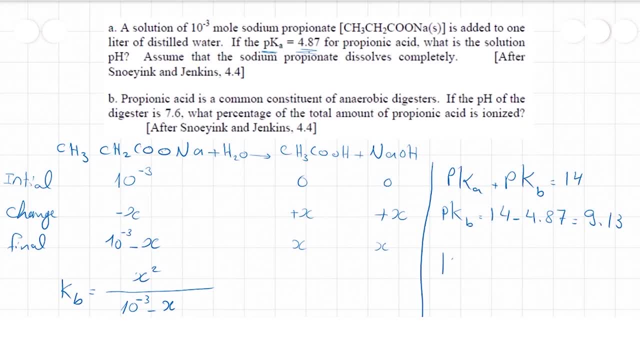 This is the value of pk. This is the value of pk, which is 4.87 equal to 9.13.. We need the value of kp, which is equal to 10 to the power minus pkp, which is equal to 10 to the power minus 9.13, equal to 7.4 multiplied by 10 to the power minus 10.. 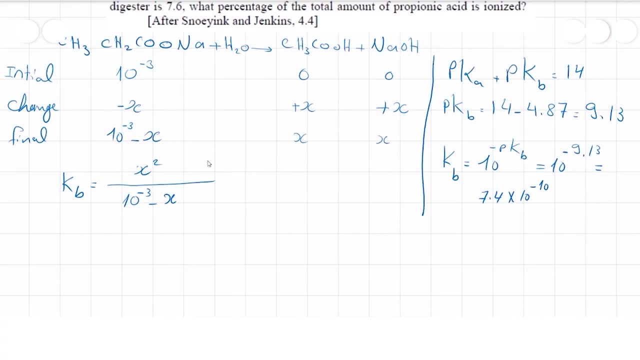 We can see this value is a very small value, so we will ignore the minus x and we will substitute here in the value of kp. So I have 7.13.. I have 7.4 multiplied by 10 to the power, minus 10, equal to x squared divided by 10 to the power. 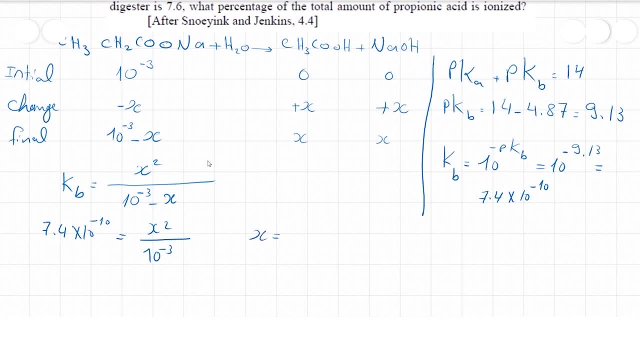 minus 3.. It will give me that x value is equal to the square root of 7.4, multiplied by 10 to the power minus 10, multiplied by 10 to the power minus 3.. The x value is equal to 8.6 multiplied by 10 to the power. 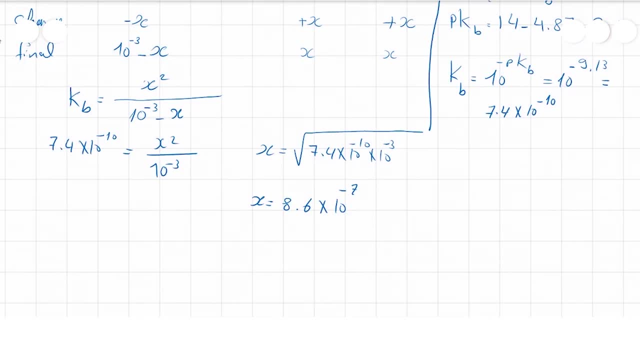 minus 7.. Remember, we need the pOH first, which is equal to minus log x, which is equal to minus log 8.6, multiplied by 10 to the power, minus 7, equal to 6.05.. From that we can calculate the value of the pH, which is equal to 14.7.. 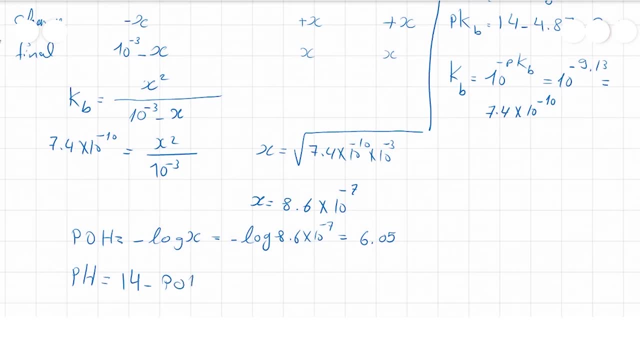 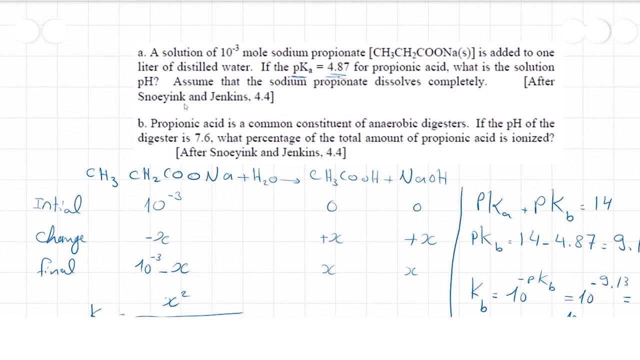 minus the value of the pOH, which is equal to 13, minus 6.05, equal to 7.94.. This is the first part of the question. The second part: we need to calculate the percentage of the total amount of propionic acid which is ionized. 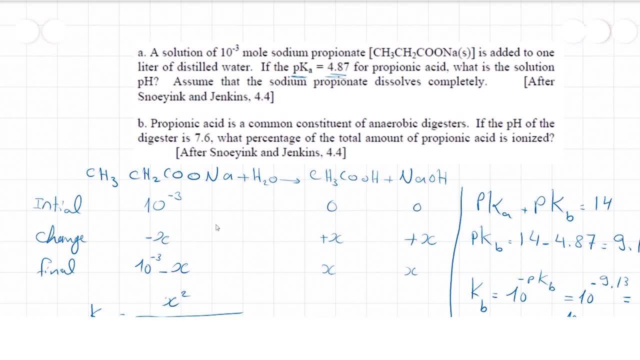 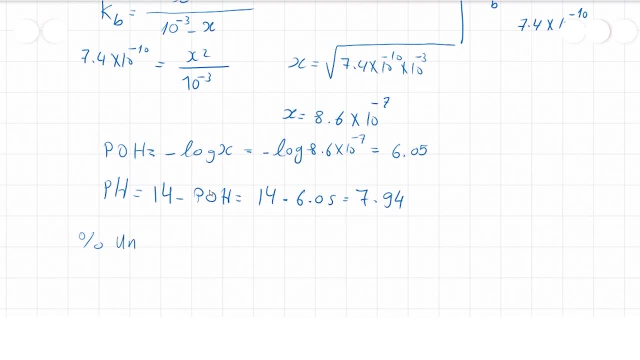 Assuming that I have, the pH is equal to 7.6.. Now first let's calculate the unionized part. The percentage of the unionized part is equal to 1 divided by 1, plus into the power of pH minus pKe multiplied by 100.